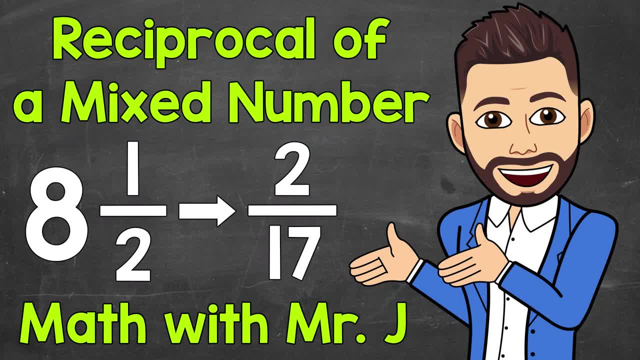 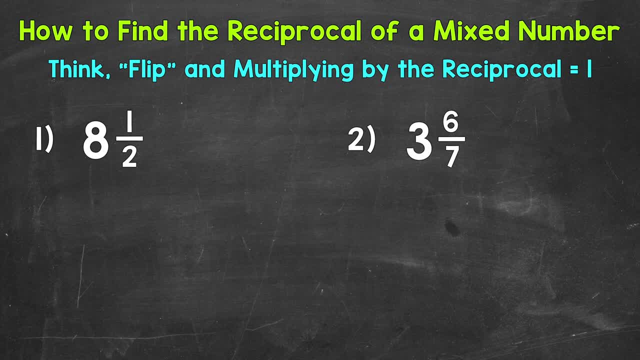 Welcome to Math with Mr J. In this video I'm going to cover how to find the reciprocal of a mixed number. Now, when we think of a reciprocal, we need to think flip and that when we multiply a mixed number or any number by its reciprocal, we get 1.. Let's jump into our examples. 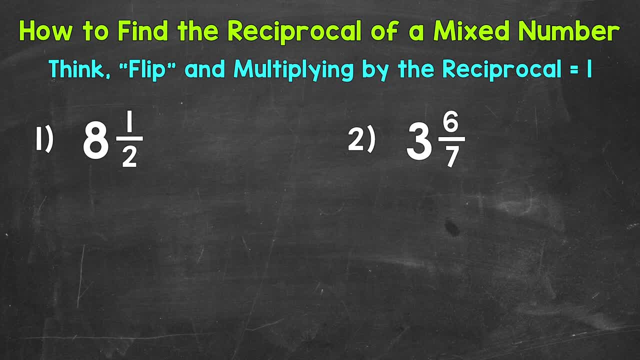 starting with number 1, where we have 8 and a half and we're going to find the reciprocal, The first thing that we need to do is to write our mixed number as an improper fraction. That way, we just have a numerator and a denominator. Once we have an improper fraction, we can flip it to. 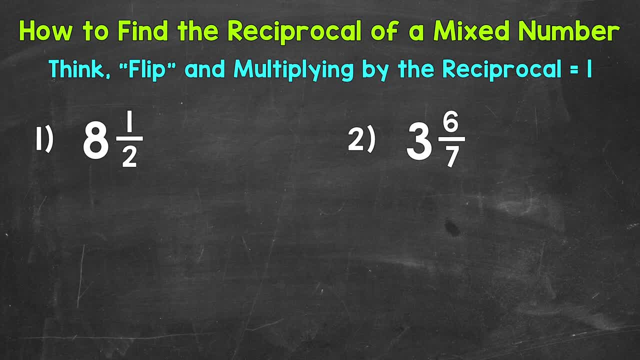 get the reciprocal, Let's multiply, then add to get our improper fraction starting at the bottom. So we start at the bottom here, We work our way up, We multiply and then add. So 2 times 8 is 16, plus 1 is 17.. So 17 is the numerator of our improper fraction. 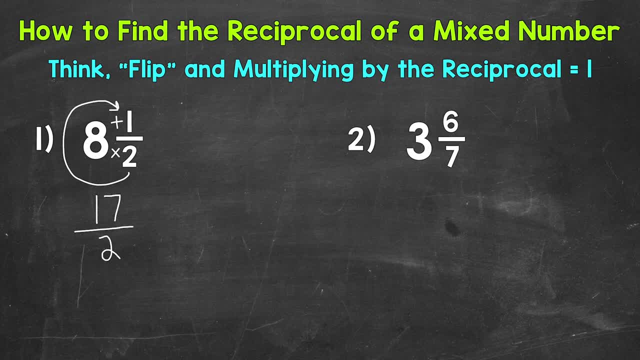 and we keep the denominator of 2.. Now that we have our improper fraction, we flip it to get the reciprocal. The denominator becomes the numerator and the numerator becomes the denominator. So we get 2 over 17, and this is our reciprocal. 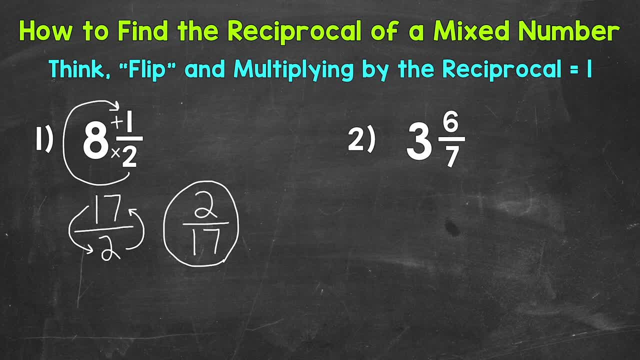 Now let's multiply the improper fraction of 17 over 2 by the reciprocal 2 over 17, to show that we get 1 when multiplying by the reciprocal. So we will come underneath here: 17 over 2, times 2 over 17,. 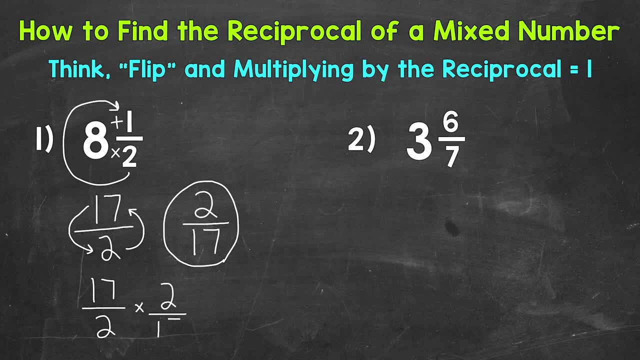 2 over 17.. And when we multiply fractions we multiply straight across. So 17 times 2, 34.. And 2 times 17 is 34.. So the same numerator over the same denominator equals one whole, which is just 1.. And we see that the original improper fraction of 17 over 2 times its. 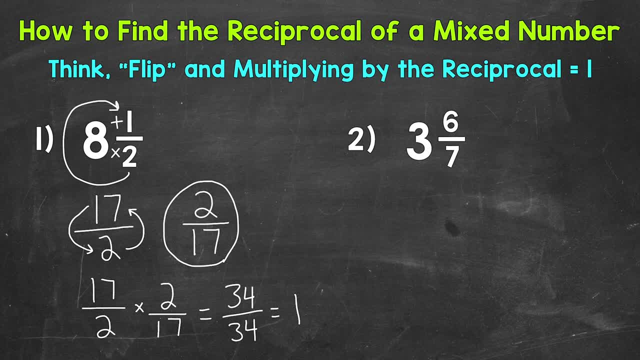 reciprocal of 2 over 17 equals 1.. So again, the reciprocal of 8 and a half is 2 over 17,, 2 17ths. Let's move on to number two, where we have 3 and 6 7ths. Again, the first thing that 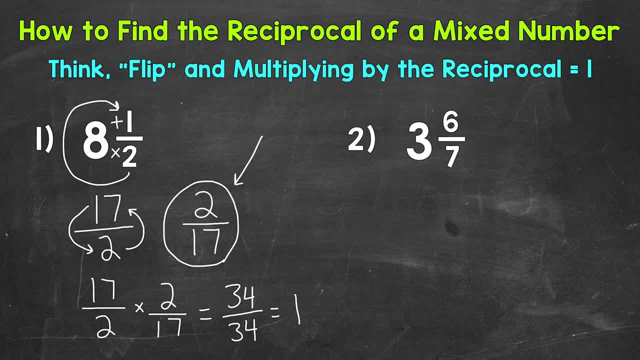 we need to do is to convert this to an improper fraction. So we multiply and then add, starting at the bottom here. So multiply and then add. So 7 times 3 is 21, plus 6 is 27.. So we get 27 over 7,, 27 7ths Now in order to get. 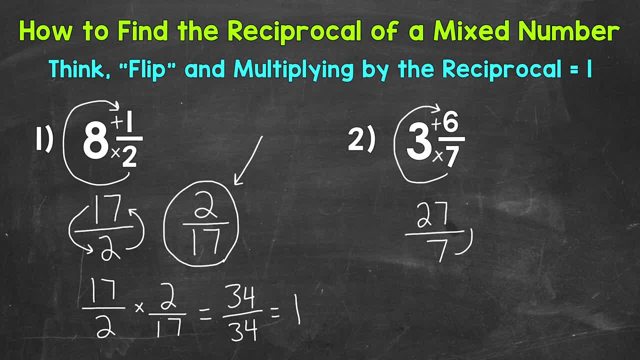 the reciprocal. we flip that So the denominator becomes the numerator and the numerator becomes the denominator. So we get 7- 27ths for our reciprocal. Now let's show that when we multiply our original improper fraction, 27- 7ths- 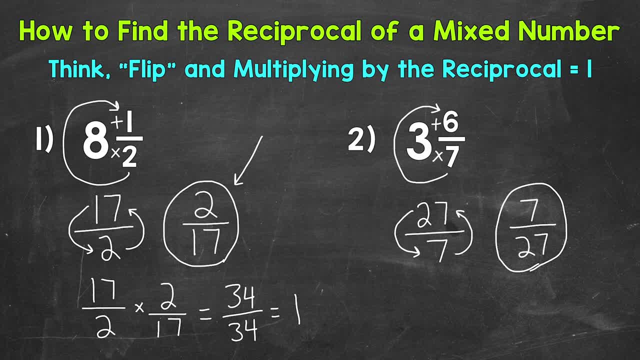 by the reciprocal that, we get one whole. So 27 over 7 times 7 27ths, 7 over 27.. 27 times 7 equals 189.. And 7 times 27 is 27.. So we get 27 7ths. Now let's show that when we multiply our original. 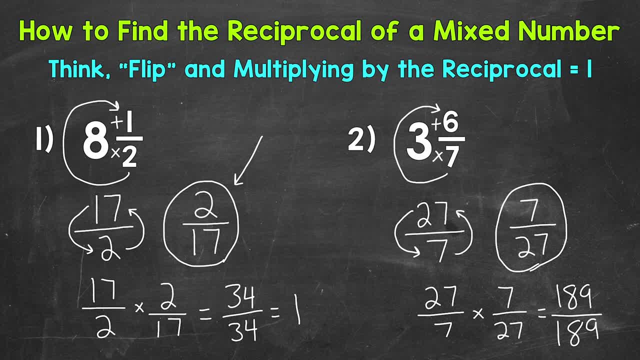 improper fraction 27 equals 189 as well. So we get 189 over 189, which equals 1.. And that shows that our improper fraction times the reciprocal equals 1.. So the reciprocal of 3 and 6, 7ths is: 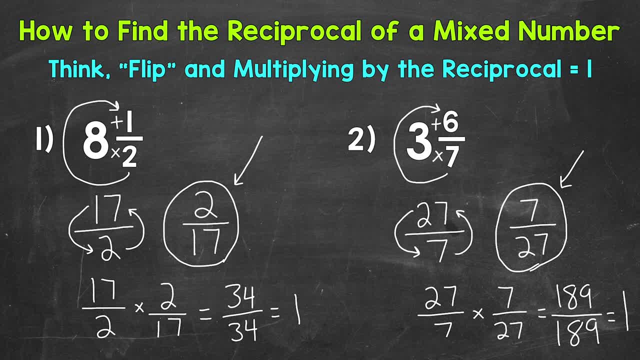 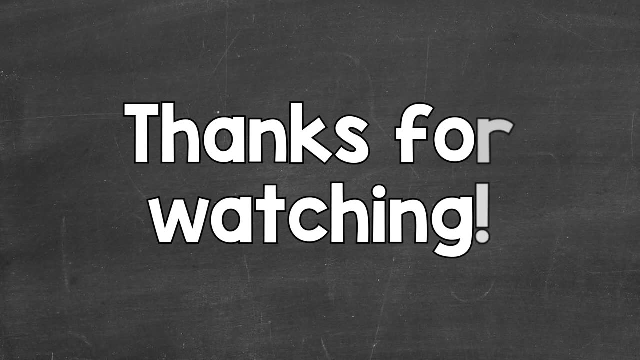 7, 27ths. So there you have it. There's how you find the reciprocal of a mixed number. Convert the mixed number to an improper fraction and then flip that improper fraction to get the reciprocal. I hope that helped. Thanks so much for watching. Until next time, peace.